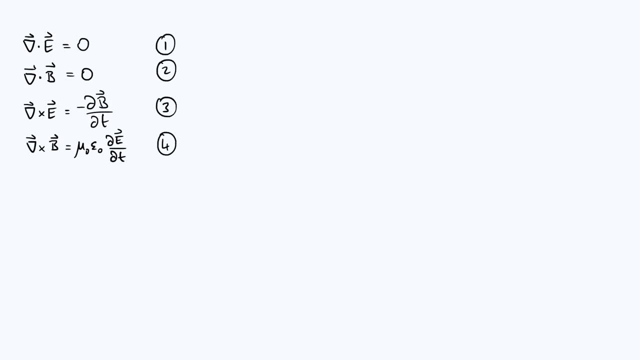 that we're going to take is basically take the curl of equation three. the right hand side will then involve curl B. we can then substitute curl B from equation four into equation three and thus eliminate B. You could do it the other way around if you wanted. you could take the curl of equation. 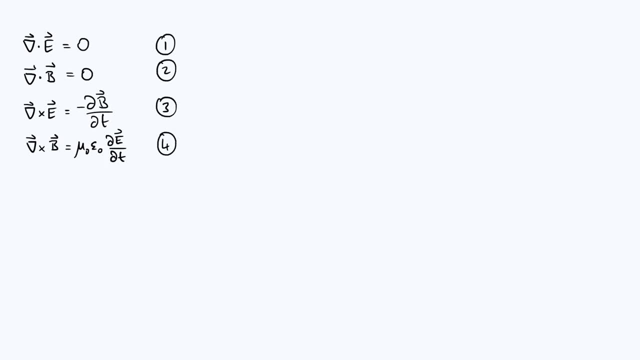 four first and then substitute curl E from three into four, but it doesn't really matter, So let's have a look at how the details are going to work. Okay, so, as we said, we are going to take the curl of the entire equation. three, So the left hand. 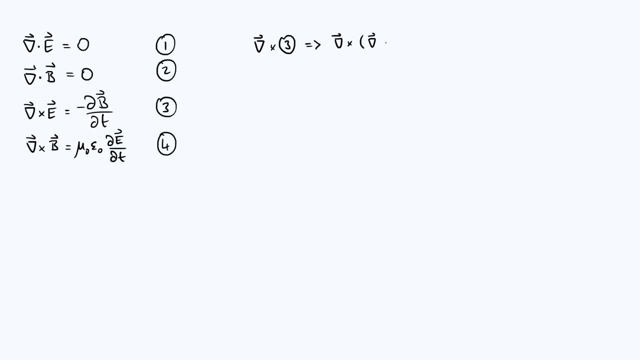 side will for now just leave as the curl of the curl of E. The right hand side is well minus the curl of DB by DT, but the operator D by DT and the curl operator can meet with each other, basically because it doesn't matter whether you differentiate with respect to time first or with respect to 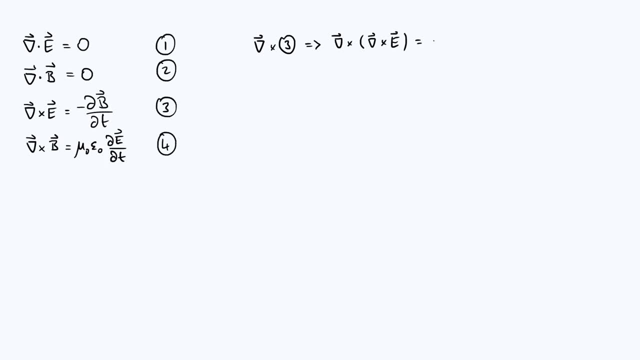 spatial coordinate first, And so I'm going to write the right hand side as minus D by DT of curl B, And then we are going to rewrite both sides in a more useful way. So we need to use some sort of vector calculus identity. I'm going to quote this here. You can look up the proof if you'd like, or 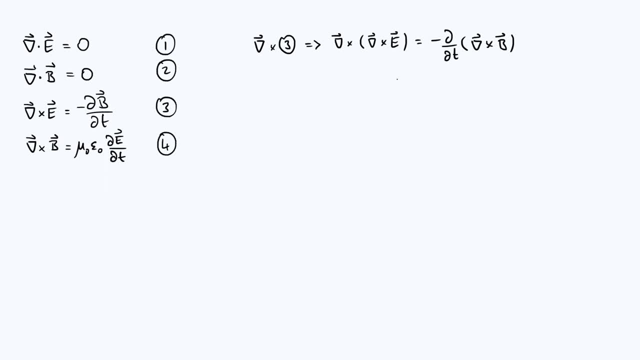 if you want to see me do a video on that, feel free to ask. But the identity we're going to use of a vector field is as follows: It is the gradient of the divergence, In other words, written like that and then minus the Laplacian of the vector field like that, And what are we? 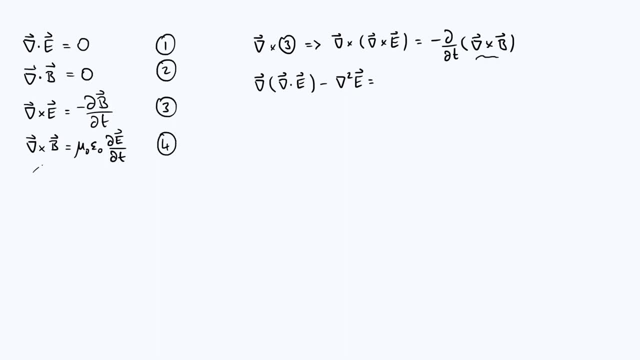 going to do with the right hand side. Well, curl B we can substitute from equation four. we can substitute that in terms of E, And so the right hand side is now minus D by DT of mu, naught epsilon naught D, E by DT. And we've already eliminated B. right Now we've got an. 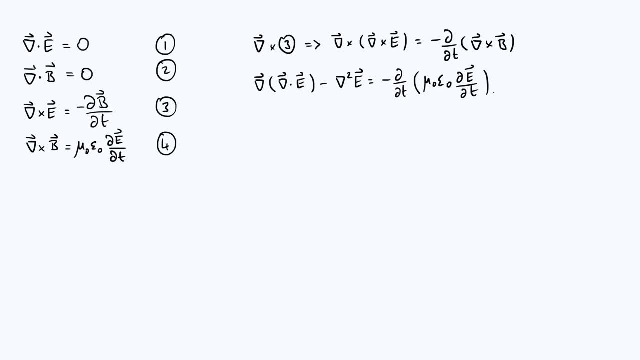 equation that only involves E. All we have to do is simplify this down and see what happens. Now you'll be able to immediately spot that we've got the divergence of E, but we know from equation one that the divergence of E is just zero, So that entire first term conveniently disappears. And 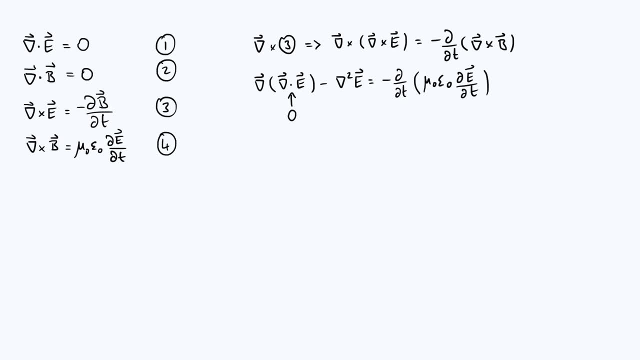 the right hand side. there's not really much we can do with that. like mu naught, epsilon naught is a constant, So this just becomes minus mu naught, epsilon naught, times D2E by DT squared. So if we just 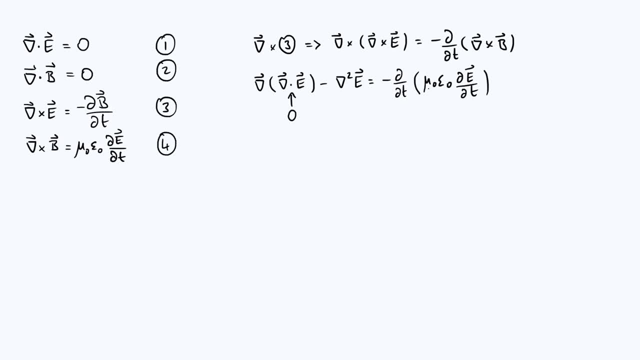 tidy that up, put all the terms on the same side. I'm also going to divide through: by mu naught, epsilon naught, You end up with D2E. by DT squared minus one over mu naught, epsilon naught times Laplacian. 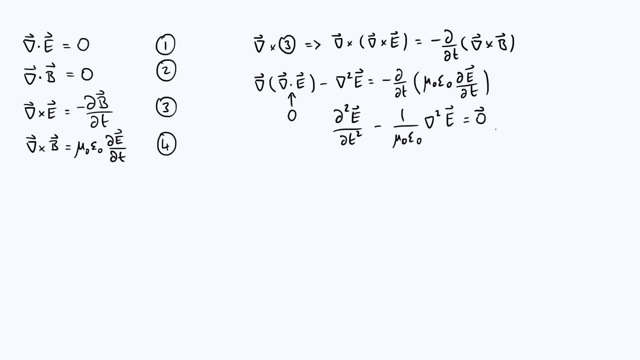 So that's the way. you know that the distance of E is equal to the zero vector. Now, the reason I've written it in this particular form is because that's recognisable as a specific case of the general wave equation. So let me note this down: We've got a wave equation, It's a vector equation. 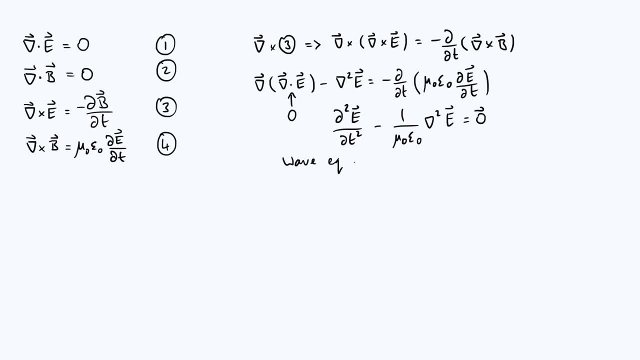 right, So it's really three wave equations. Each individual component of the electric field oscillates according to the wave equation, But it's a well-established result that that coefficient in front of DL, squared E, is the squared velocity of the waves. right, So we can say the speed of. 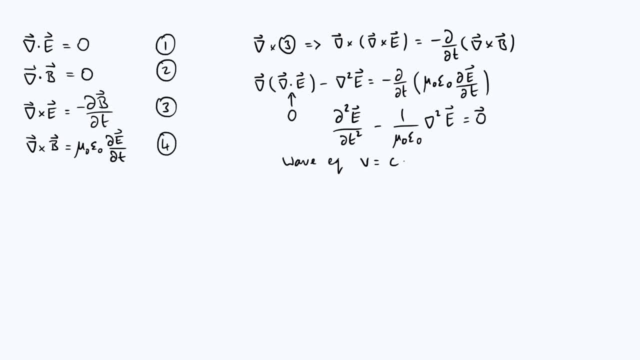 the waves V, which is of course the speed of light, because these are electromagnetic waves, so we can call that C is one over the square root of mu naught, epsilon naught. So we've already got our first, very interesting result, which is this relationship between three. 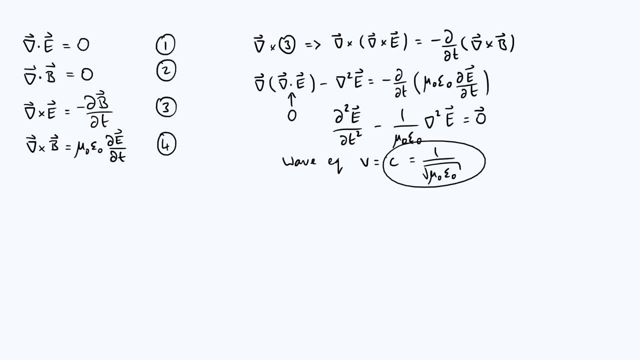 fundamental constants right: Speed of light and mu naught and epsilon naught. So so far what we showed right is that each against 0.. But here we also know that the force at which the weight of the vector drops viscerally is quadşekkürally greater than mu naught times E into the 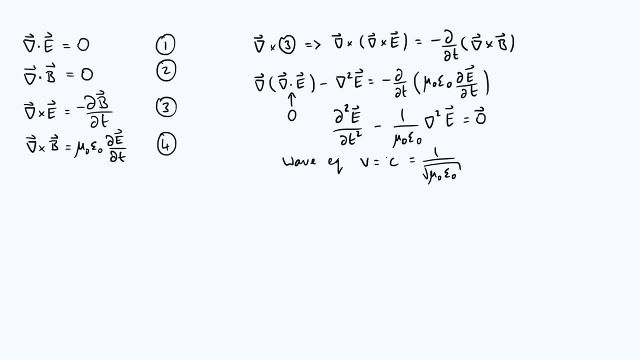 force of the vector, which is given through experience and concussion problems, is now not the frequency of the component of the electric field obeys the wave equation. now, just to make that a little bit more concrete, let's actually write down an expression for the electric field that comes from that wave. 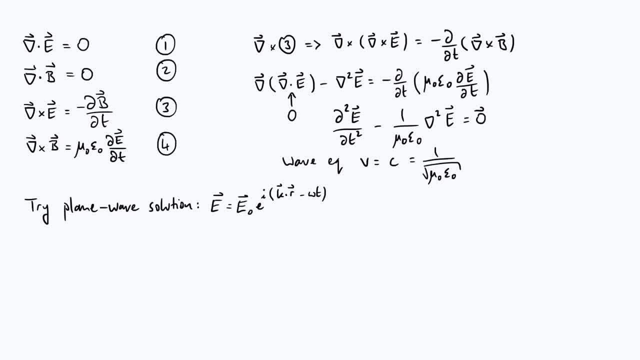 equation, and we're going to do this basically just by getting a sensible solution and substituting it in. and we already know it's a wave equation and so a sensible thing to do, as i've written here, would be to try a plane wave solution, and plane waves take this kind of form here. this e naught. 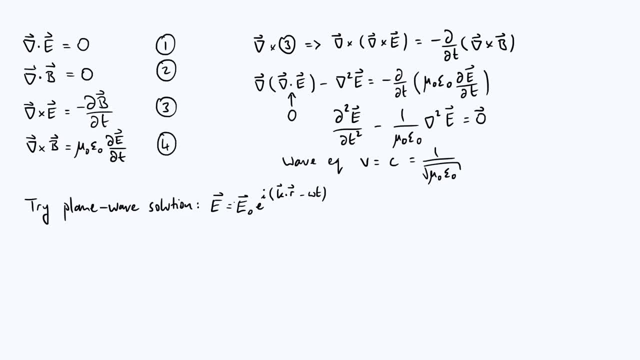 is kind of like the amplitude, but remember it's really a vector. so the three components of e naught are telling you the amplitude of oscillations of your electric field in the three different coordinate axes, and k is the wave vector that tells you the direction that the wave is moving. 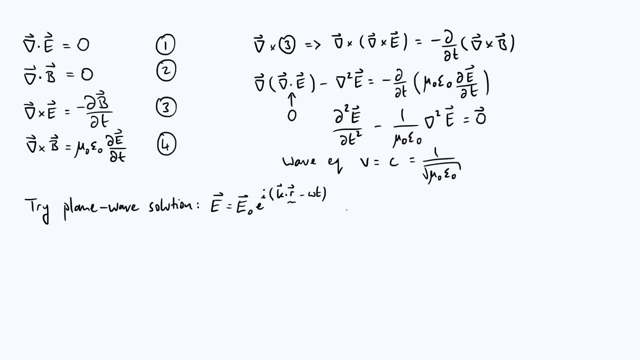 in. r is your position vector and omega is the angular frequency, so this is a plane wave solution. let's substitute that into the wave equation and see what happens. well, with this second time derivative. each time derivative is a wave equation, and so this is a plane wave solution. 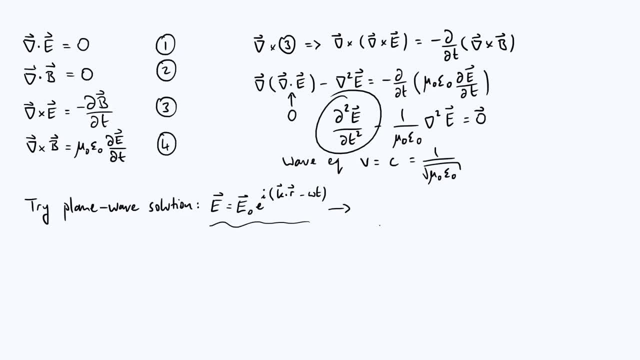 and so this is a plane wave solution. and so this is a plane wave solution. you differentiate this thing with respect to time. you're just going to pull down a factor of minus i omega- right, because you've got an i here minus omega, and then that's all multiplied. 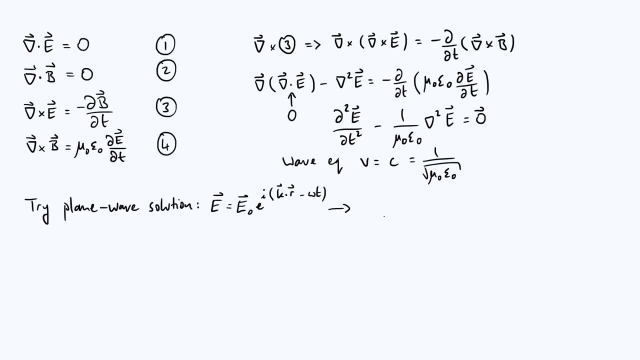 by the t. so if we do i well, minus i omega times, minus i omega one for each of the time derivatives, you get minus omega squared. so that bit there is minus omega squared, uh, multiplied by the original electric field, e, and then you get minus omega squared, and then you get minus omega squared. 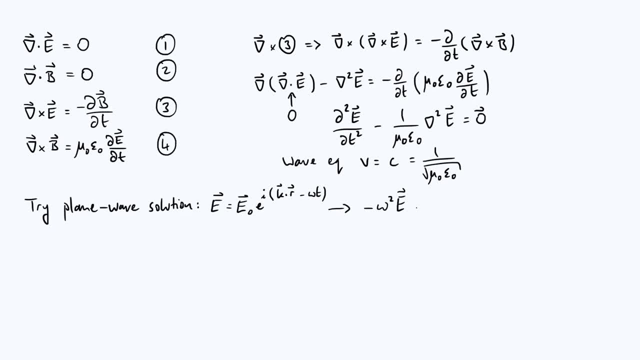 and what about this um laplacian? well, okay, let's start by writing in minus c squared for this one over mu naught, epsilon naught bit um the laplacian, remember, is the second derivative with respect to x, plus the second derivative with respect to y, and then the same uh for z. now, if you imagine, 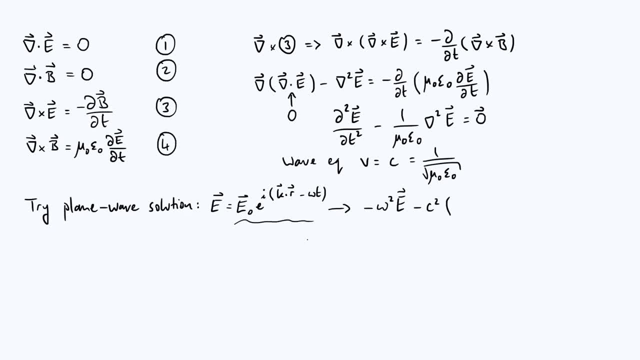 differentiating your electric field with respect to x. you are going to pull down a factor of ikx, right? i mean ik subscript x, where kx is the x component of your wave vector k. so if you do that twice you get that whole thing. it's. 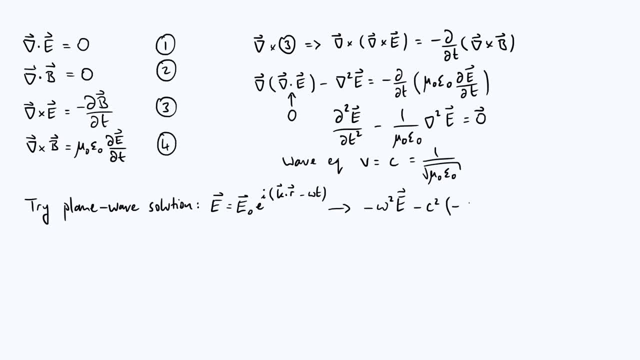 squared, and i squared is minus one, and so you get a factor of minus kx squared, and then, of course, identical method for the y and z derivatives. so i get minus ky squared, minus kz squared, all of that multiplied by the original electric field, and that's supposed to be the zero vector. um, now the 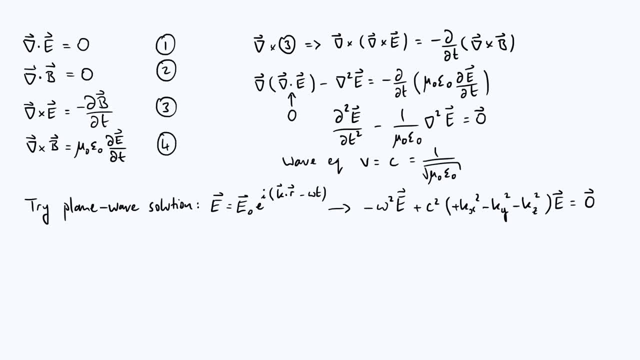 conclusion here is that you get minus kx squared, minus kz squared, and then you get minus kx squared, and then you get minus kx squared, minus kz squared, and then you get minus kx squared minus kz squared. i guess we can, uh well, we may as well change all of these to positive signs, because we've got a. 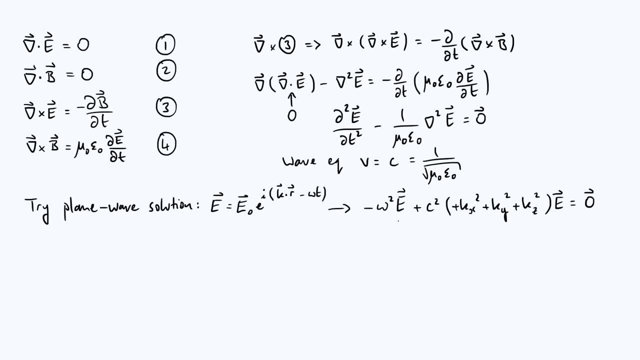 double minus, and the conclusion is: because both of these terms are proportional to the electric field. this thing here has to be equal to all of this if we want to get the zero vector, and we conclude that omega itself has to be c times. uh, the modulus of the wave vector k. um, that's come. 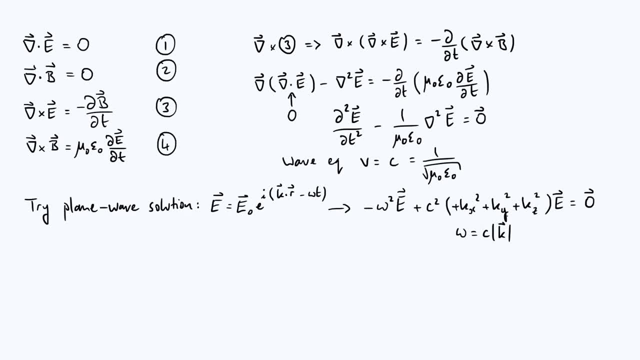 from square rooting, all of this stuff. like if you square k- sorry, if you square root k and you square kx squared plus ky squared plus kz squared, you get the modulus of k right. so we've derived um from our wave equation, the relationship between angular frequency and the size of the wave vector. 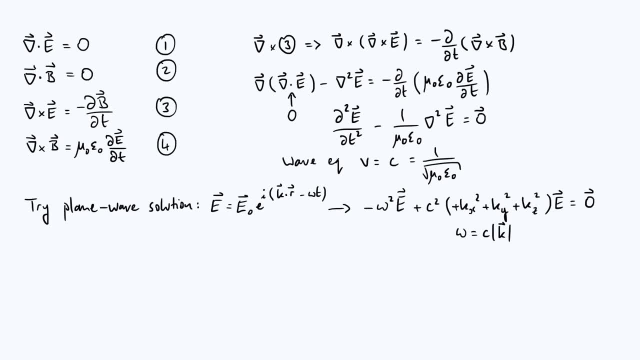 so we've got our plane wave solution for the oscillating electric field. now we want to see how the magnetic field behaves and um sort of investigate how, uh, the e and b fields are related to each other. now there are different ways to do this. the approach i'm going to take is to use equation 3 because we already have an you can borrowed from elsewhere- were x and y and z vectors expression, and so each of these got the same rate and the value of x and y and z values and the power of x and y. you can also go back to this exercise where we've got a flat sheet right here, so we divide the. 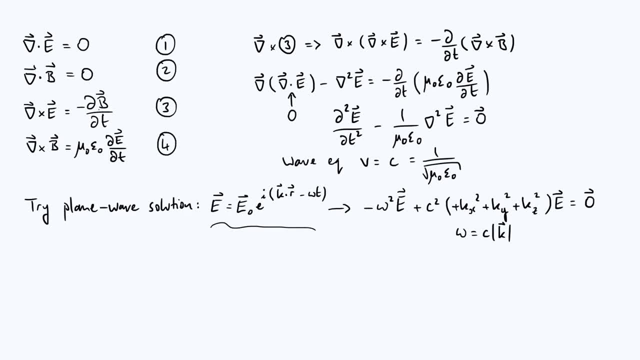 probability of this equation by the positive number of ng. we'll produce out this equation from the comma here, and this equation, يا power, will indicate that now, if you do better, you should for e. so we could substitute that into equation three and then integrate it with respect to time. 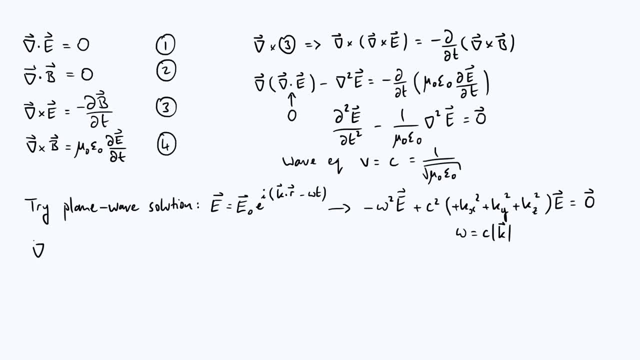 to find the b field. So the first thing I'd like to do is find curl of e, given that we know that a solution for e looks like that plane wave, And so I'm going to write this as the curl of the vector amplitude e naught, and I'm going to abbreviate the complex exponential as e to the i. 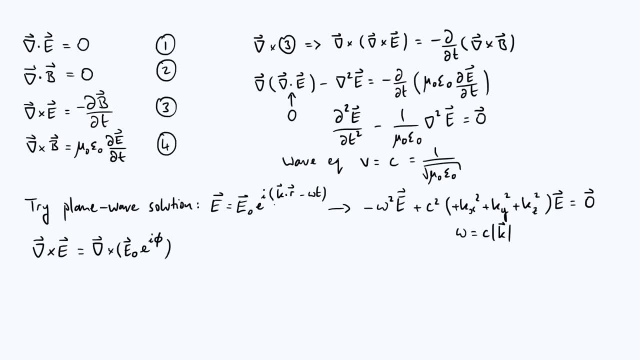 phi, where it's sort of understood that the phi is k dot r minus m a t. just to save a little bit of space, save a little bit of writing Now, e naught is a vector, e to the i phi is a scalar. 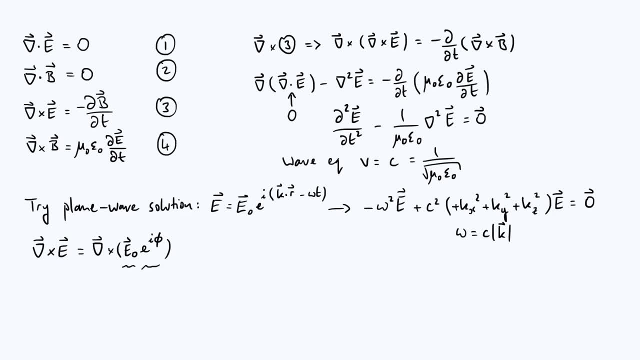 and e to the i. phi is really a scalar field because it depends on x, y and z via the position vector r, right? So we're taking the curl of a vector times a scalar, And so we can use another vector, calculus identity, to do that. 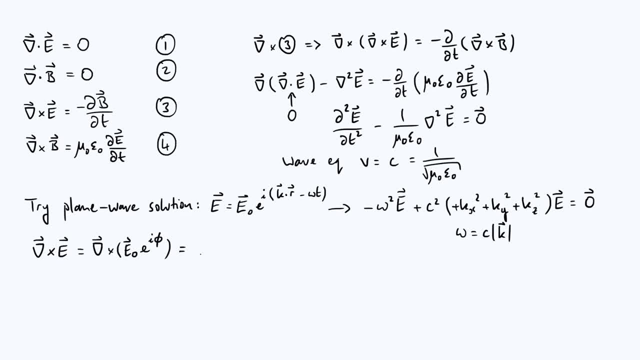 Again, I'm not going to prove this here. Let me know if you'd like to see a proof, But for now I'm just going to quote that the curl of a vector times a scalar is the gradient of the scalar right. 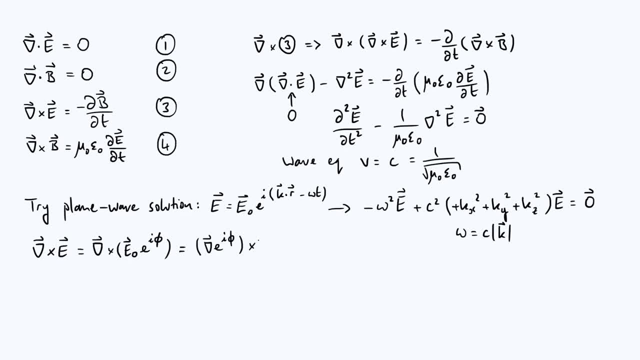 So, grad of e to the i phi crossed with the vector which is e naught. Well, and then we have to add on the scalar which is e to the i phi times the curl of the vector which is curl of e naught. 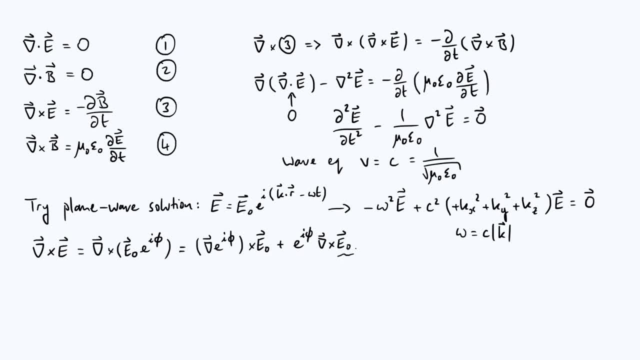 Now something nice happens in this particular case, because e, naught is a constant and doesn't therefore actually have any spatial derivatives. So the curl is just zero, and we only get this this first term here. The next question is: how does the gradient operator act on e to the i? 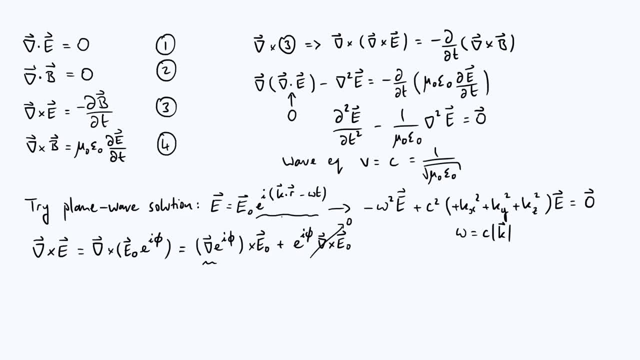 Phi, which is this bit here, Well, the gradient operator, remember just the vector of three spatial derivatives. When we differentiate e to the i, phi with respect to x, the coefficient of x. because of this dot product, the coefficient of x will be the x component of the wave vector k. 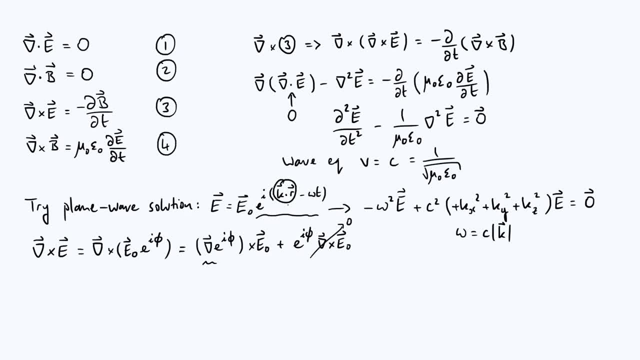 And so the x component of the gradient vector will basically just multiply your, your original scalar, by i times kx, And you can Make the same argument for the y and z components. right, You differentiate e to the i phi. with respect to y, you pull down a factor of i ky. differentiate with respect to z: you pull down a factor of i kz. 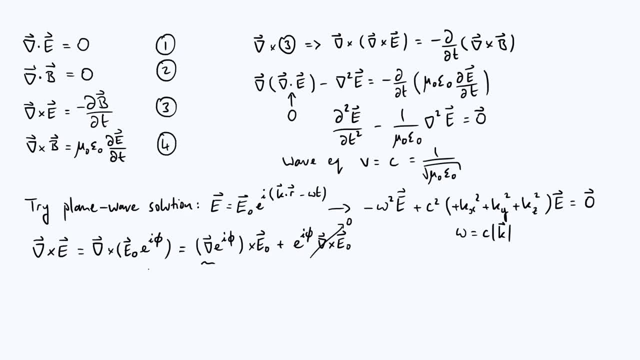 And so this gradient vector here is actually just equivalent to multiplying the whole thing by i times the wave vector k, So I can write that as i k e to the i phi crossed with e. naught Like that Now, because e to the i phi is a scalar and the cross product is 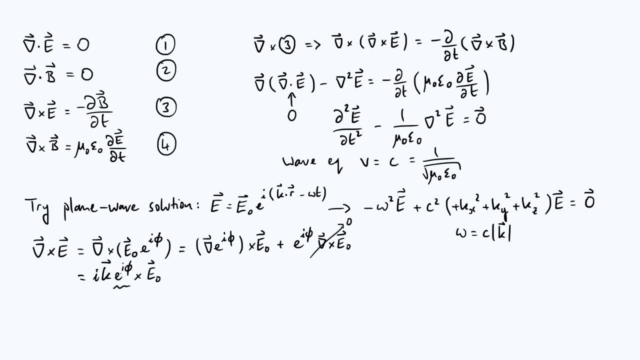 linear in both of its vector arguments. doesn't really matter whether we put the e to the i phi there or after the e, nor so what we could do is imagine putting the e to the i phi at the end. then you would have e naught, e to the i phi, which is just the electric field. 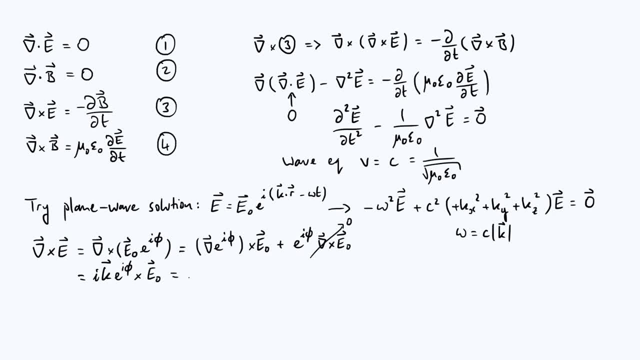 E right, And so I can write this curl of e as i k crossed with the e Vector itself. Now, what can we conclude from that? Well, we go back to equation 3.. Equation 3 then tells us that the time derivative of b db by dt is minus. ik cross e right. 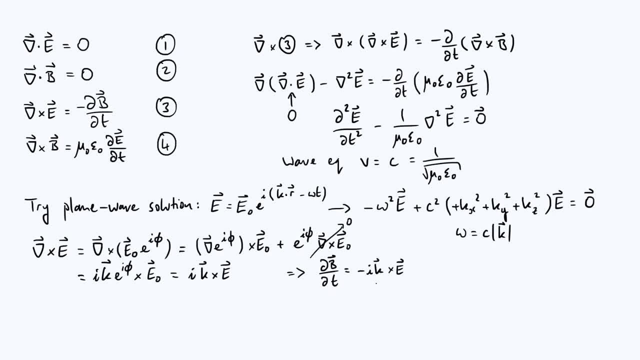 All I've done there is substituted curly equals, ik cross e and then we can integrate both sides and say that the magnetic field b is minus. ik crossed with the integral of the electric field with respect to time. It's pretty straightforward to do that electric field integral, actually because we already know the electric field in terms of time. 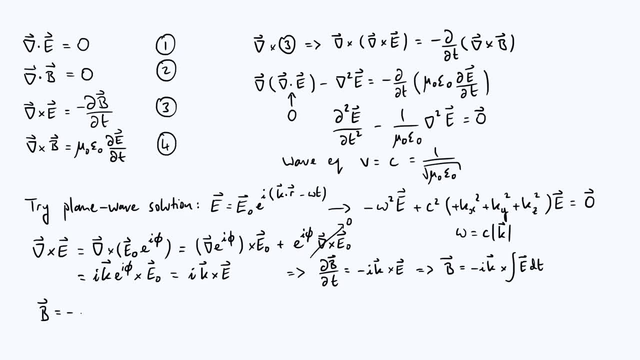 So let's go ahead and do that. So your b field is minus, ik crossed with. Well, we're trying to integrate that circled term there. The only time dependence is in the exponent in the form of minus i, omega, t. When you integrate an exponential like that, you end up just dividing by the coefficient of t. 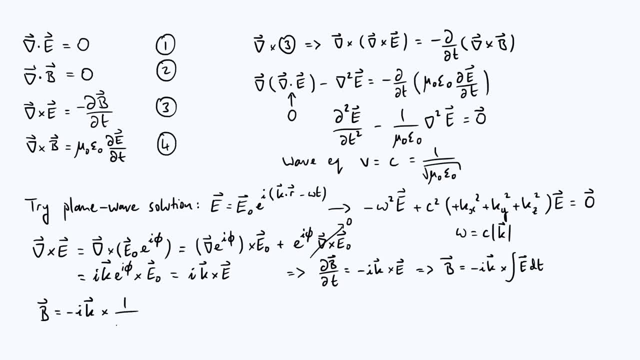 And so we're going to simply get 1 over minus i omega times the. Well, the whole thing e north, e to the, i phi Like that, And the minus i's cancel and we can tidy this up a little bit. 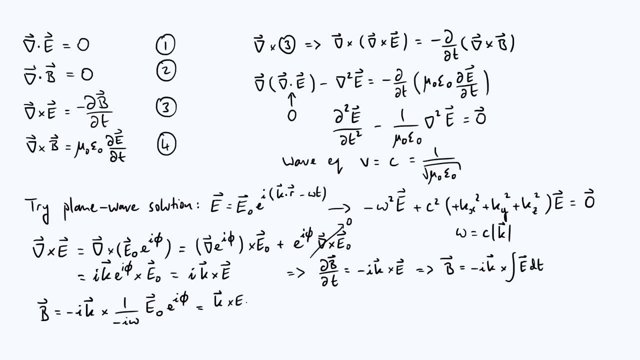 Write it as: k crossed with e north, divided by omega times e to the i phi. Now k cross e north over omega. that's just some constant vector, So we could relabel that And I guess, for self-explanatory reasons, I'm going to call that b north, right. 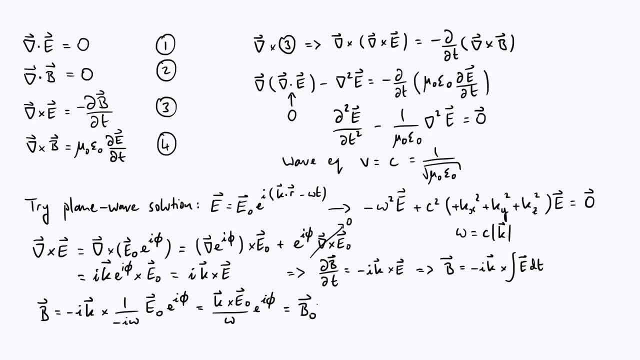 It's like. It's like the vector amplitude of our oscillating b field, So let's call that b north. It's defined as k cross, e, north over omega, And so your magnetic field solution looks like b north, e to the i phi. 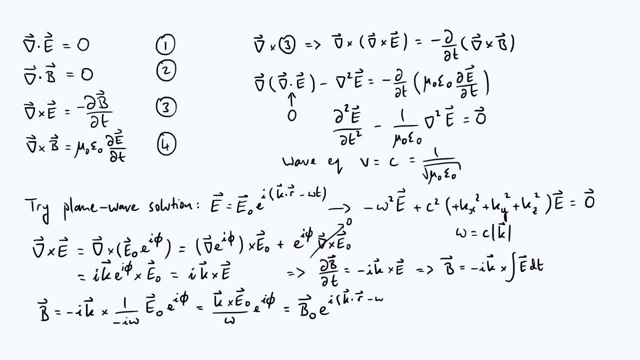 And if we write phi in again, remember it's k dot r minus omega t. So we've concluded that since the electric field is oscillating as a plane wave, the magnetic field has to do the same thing. Now you can see from the fact that you've got the same. 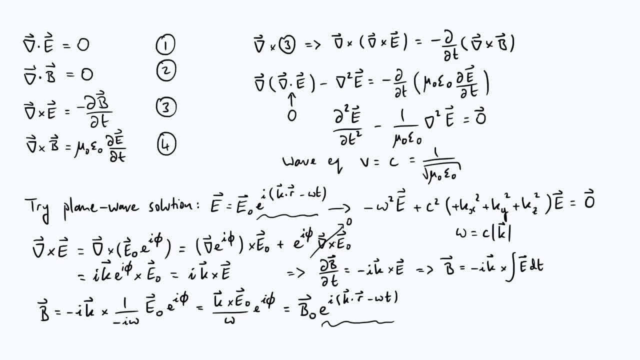 You've got the same complex exponential bit in your oscillating b field as you do in your oscillating e field, that that implies that the magnetic field wave and electric field wave have the same wave vector and the same angular frequency and that they're in phase with each other, right? 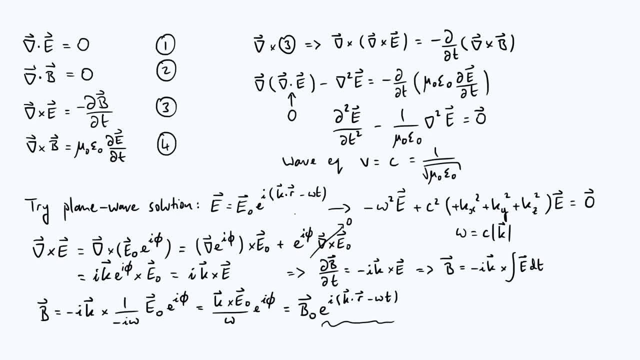 So that's an interesting conclusion. But we can also conclude something else by examining this cross product here. So the other conclusion we can make is, because b north is just this cross product divided by omega, that the b north vector has to be perpendicular to both the wave vector k and also the electric field vector e north right. 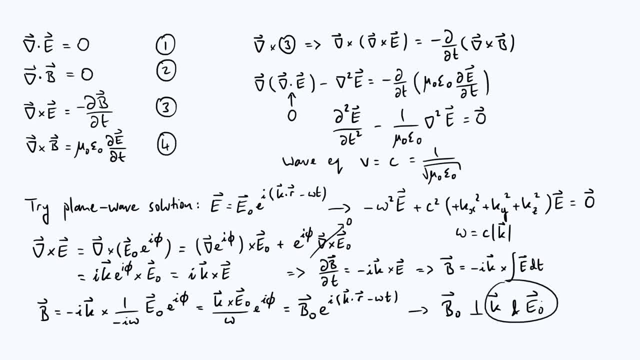 That's. We'll say a little bit more later on about how k and e north are related to each other, But for now we conclude that whatever k and e north are, b north is perpendicular to both of them because of that cross product. 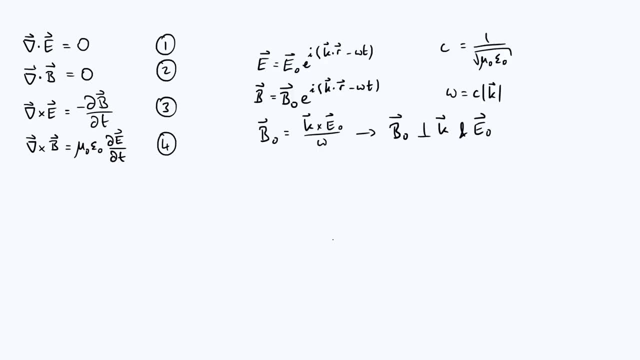 And let's just take a moment to summarize the key results that we've got so far. We've concluded that e and b Both have plane wave solutions with wave vector k, angular frequency omega. The speed of those waves is the speed of light given by one over root. mu naught, epsilon naught. 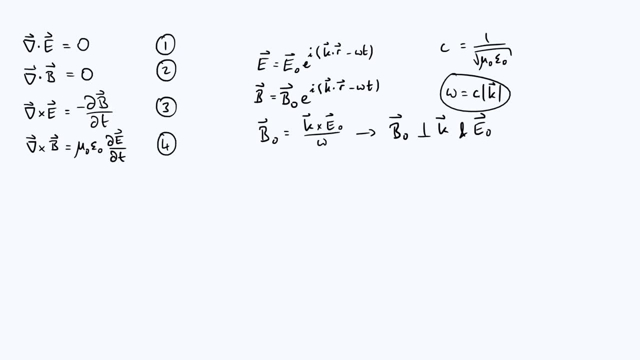 And omega and the modulus of k are related by omega equals c times mod k. And the electric and magnetic fields are not independent of each other in the sense that, well, firstly they have the same wave vector and frequency, but also the amplitudes have to be related by. 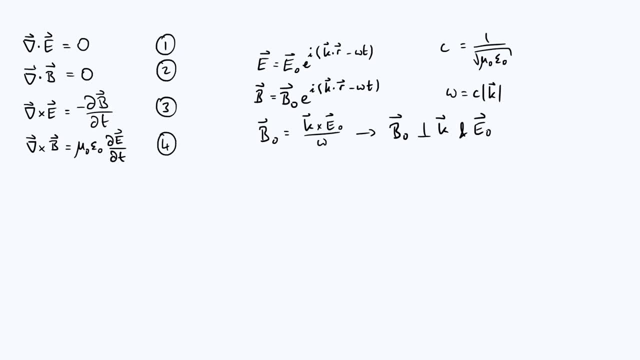 this Equation here, which tells us that the magnetic and electric fields are perpendicular, and also that the magnetic field is perpendicular to the wave vector. Now, the missing piece really is that we haven't said anything about how k and e north are related to each other. 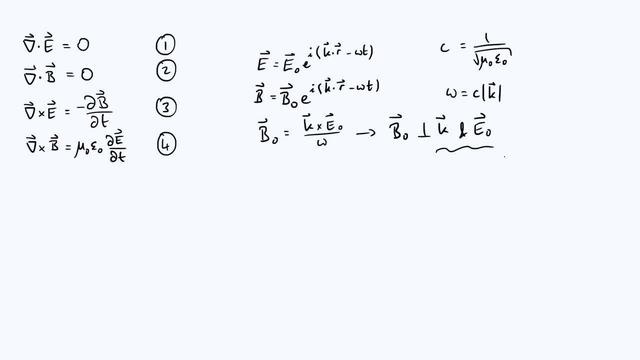 There is another constraint on the behavior of these waves, which comes from equation one, the divergence of e having to be zero. Let's consider what the divergence of e actually is, given that we know e takes this plane wave form, And let's write it down here. 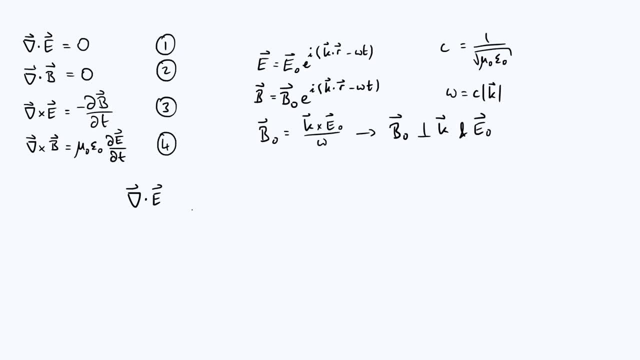 So the divergence of e. you're going to take the x component of e, differentiate it with respect to x, and then take the y component of e, differentiate it with respect to y, and the same for z, and you're going to add all of those together. 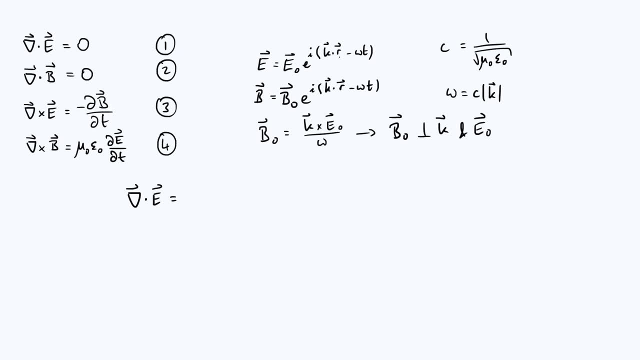 Now, when you differentiate with respect to x, for the same reasons that we were talking about earlier, you will pull down a factor of ik subscript x from that complex exponential, And so the first term in your divergence is going to be x. So that's going to be ik subscript x times the x component of e north times your complex exponential. like that: 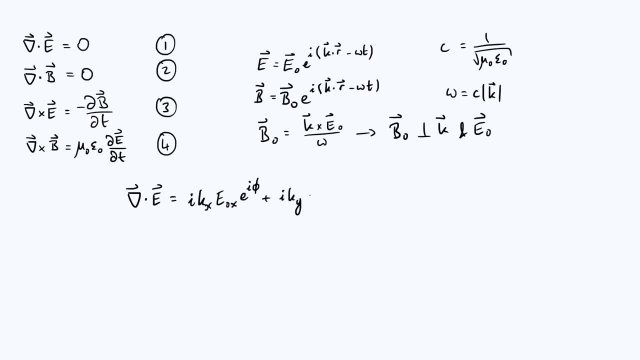 And then we're going to get identical looking terms for y and z. So iky, e, zero, y component, same phase factor, And of course, ikz from the z derivative, e north z from the z component of e north times, e to the i. 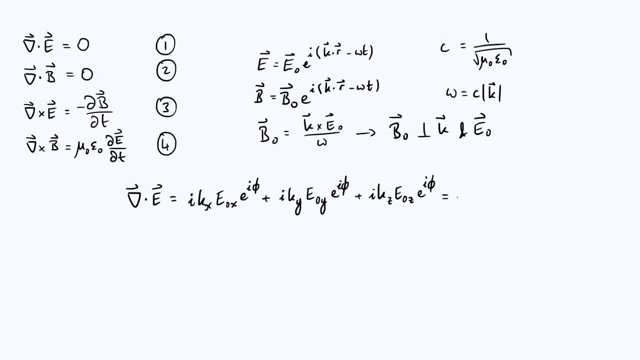 This can be written very nicely in compact vector notation as just ik dotted with e, north times, e to the i, phi And equation one says that this is all supposed to be equal to zero. Now this phase factor can't be equal to zero or is not identically equal to zero. 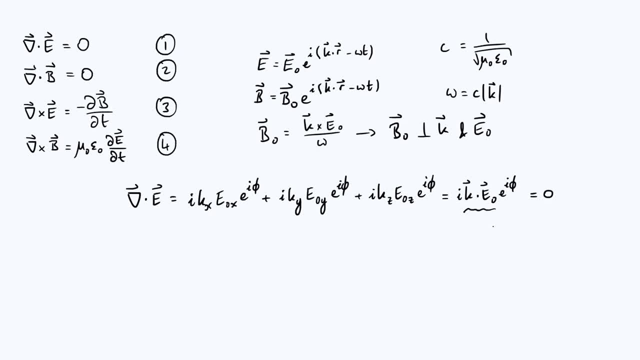 Right. And therefore k dotted with e north must be identically equal to zero. And the conclusion from that: if the dot product of vectors is zero, they're perpendicular right. So e north is perpendicular to k, And putting that fact together with the fact that b north is perpendicular to both k and e north, 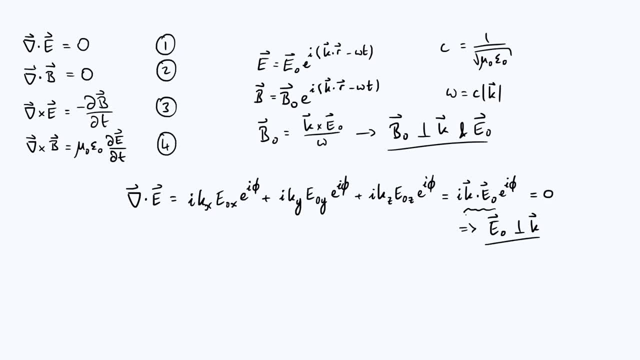 you conclude that the vectors k, the wave vector, and b north and e north, the magnetic and electric field vectors, they're all perpendicular to each other, mutually perpendicular. So if we were to draw that on a diagram, let's say your wave is propagating to the right. 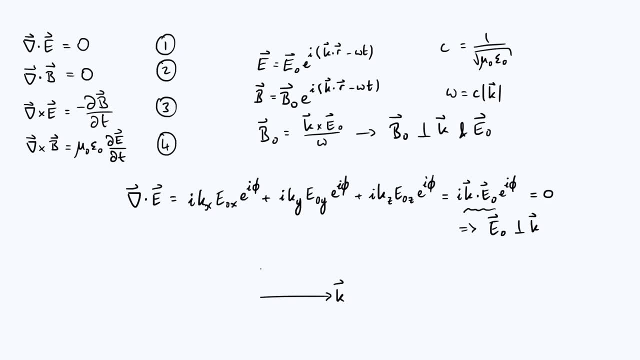 So your wave vector k looks like that And your wave vector not wave vector. your e north vector the direction of oscillation of the electric field is pointing up. Then b north would have to be either going into the page or out of the page. 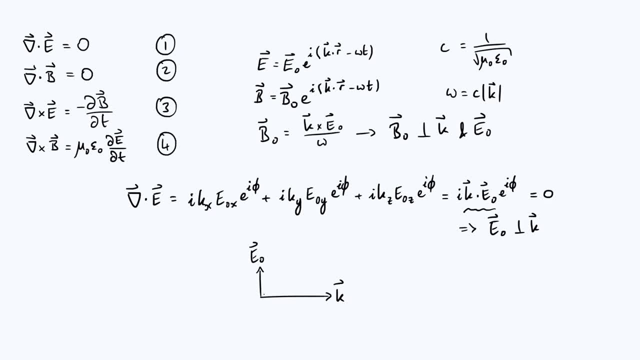 I guess I should say screen into the screen or out of the screen. We can actually decide using this cross product here, right k, cross e, north, divided by omega, And you can use whatever method you like the most To work out the direction of cross products. 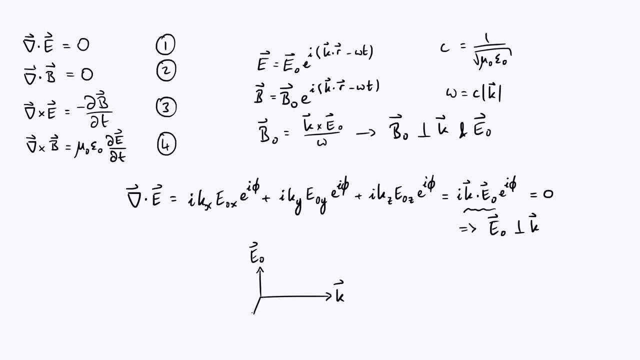 I use the right hand rule, which tells me that b north should actually be coming out of the page like this, So they're all mutually perpendicular to each other. There's actually one final conclusion we can make about the nature of these waves, given all of these results that we've got. 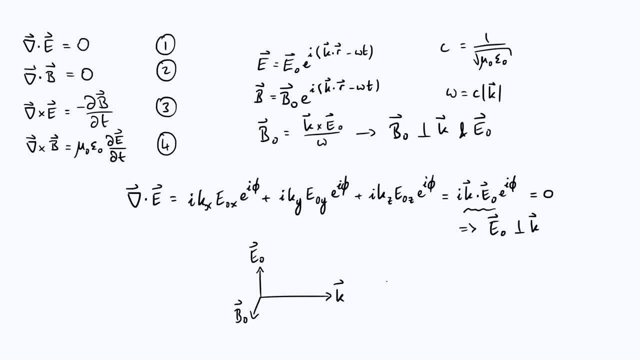 And that concerns the magnitude of e north compared with the magnitude of b north. Now, if k and e north are perpendicular to each other, then the magnitude of the cross product is just the magnitude of k times the magnitude of the wave vector. 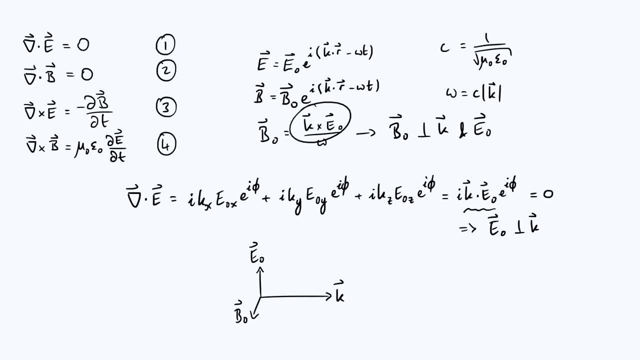 And the magnitude of e north is just the magnitude of e north right. And so from this circled equation there you conclude that the magnitude of b north is the magnitude of k divided by omega times the magnitude of e north right. There's no sine theta factor or anything, because all of our vectors are perpendicular. 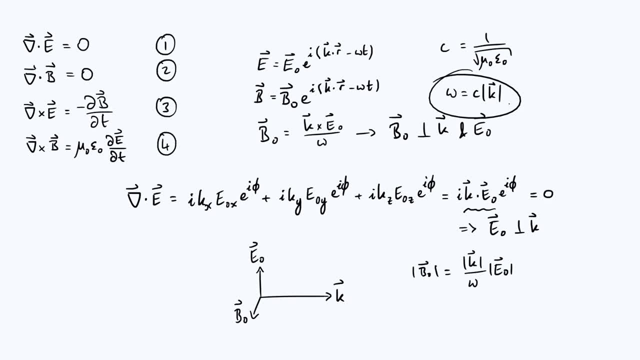 But we also know from this circled relationship up there that modulus k divided by omega is the magnitude of e north. So we conclude that the magnitude of e north is the magnitude of k divided by omega is one over c. So we conclude that the size or the amplitude of the magnetic field oscillations is the amplitude of the electric field oscillations divided by the speed of light. c right. 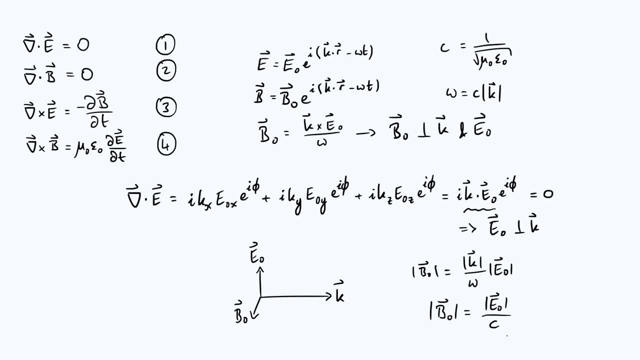 And so that's another constraint that these waves have to obey, Like the amplitudes of b and e are not independent of each other, and the ratio is always equal to c, or one over c, depending on which way around you do it.